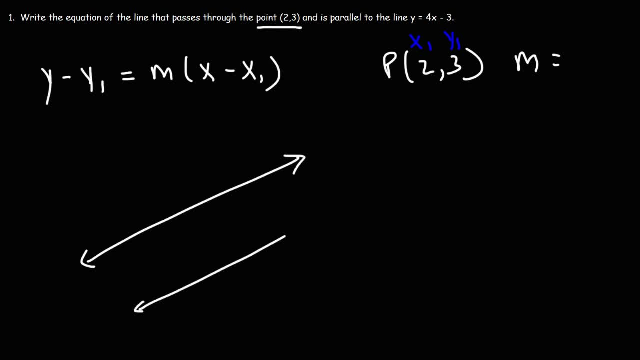 So what do we know about two parallel lines? Two parallel lines have the same slope. If the slope of the first line is 1 and the other line is parallel to it, the second line will have the same slope. So the question is: what is the slope of this line? 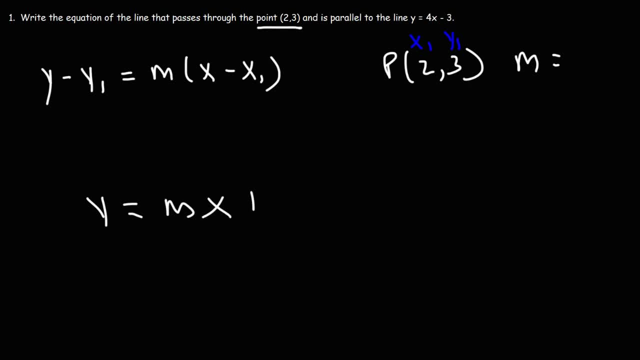 And that line is in slope-intercept form. y equals mx plus b. m is the slope, b is the y-intercept. So we have: y is equal to 4x minus 3.. So we can clearly see that the slope is equal to 4.. 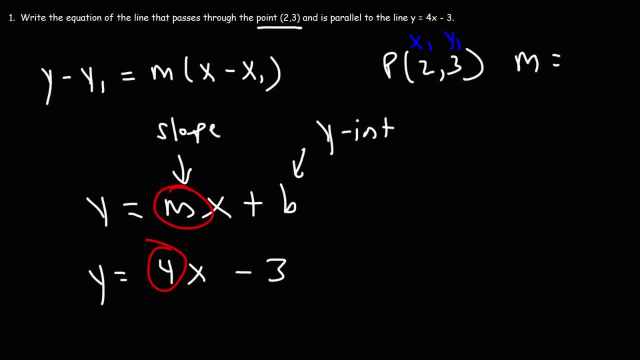 And because the lines are parallel, the slope of the line that we're trying to find is also equal to 4.. So, remember, parallel lines have the same slope. So, now that we have a point and a slope, we can now use this formula to write the equation. 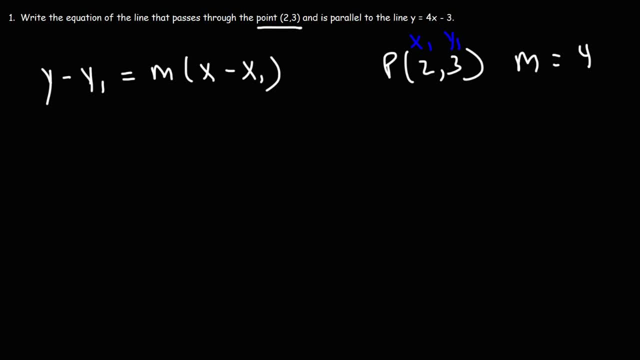 The equation of the line. So let's go ahead and do that. Let's replace y1 with 3. And then let's replace m with 4. And x1 with 2.. So this, right here, is the equation in point-slope form. 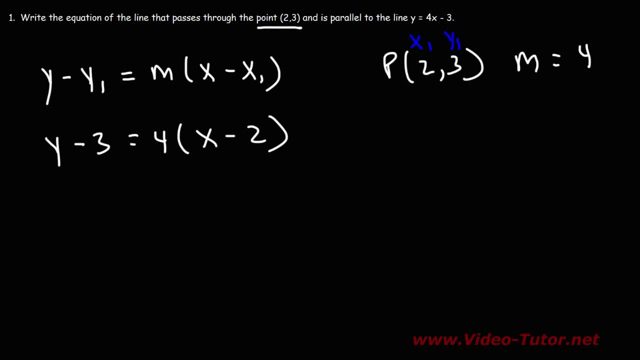 But let's get the equation in slope-intercept form. Let's solve for y, So let's distribute the 4. 4 times x is 4x, And then 4 times negative: 2 is negative, Negative 8.. Next let's add 3 to both sides of the equation. 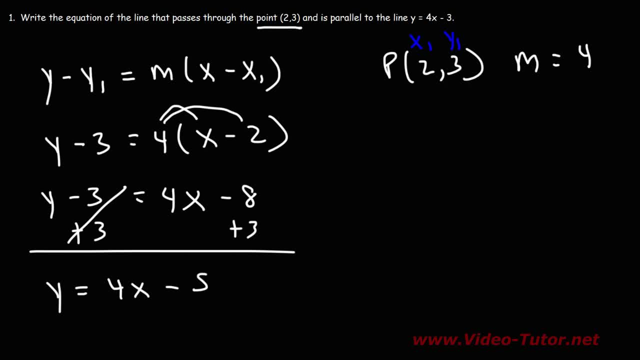 Negative. 8 plus 3 is negative 5.. So this is the answer. That is the equation of the line that passes through the point 2, 3.. And it's parallel to the line. y equals 4x minus 3.. 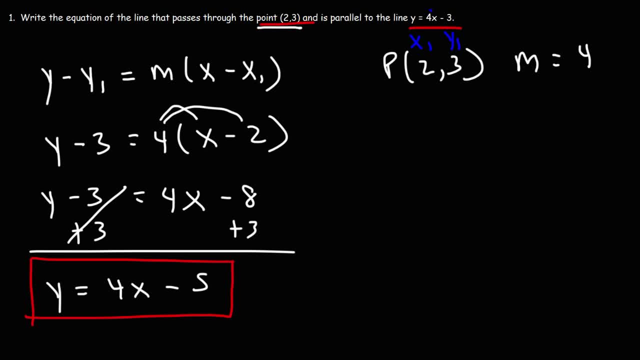 Let's think about it. We know that it's parallel to that line because these two lines have the same slope, As indicated by the term 4x. They both have a slope of 4.. Now this line contains the point 2, 3.. 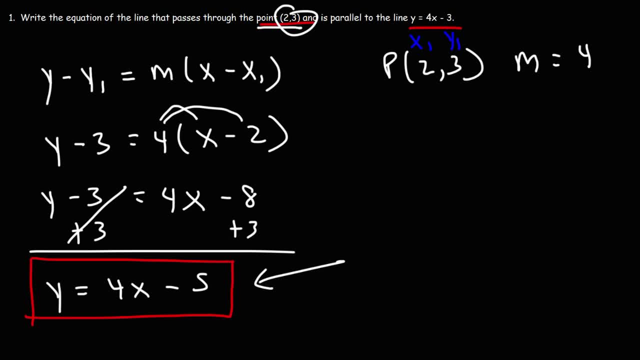 If I were to replace x with 2, I would get a y value of 3.. And we could check it 4 times 2 minus 5.. 4 times 2 is 8.. 8 minus 5 is 3.. 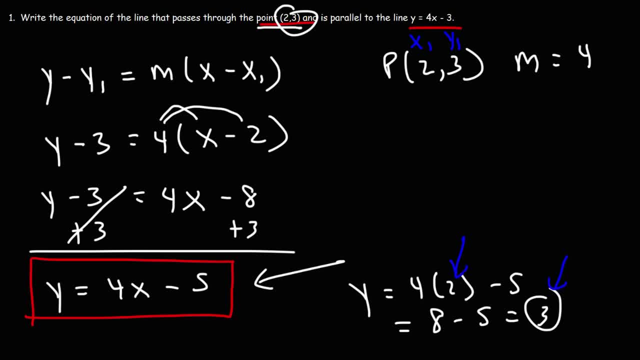 As you can see, when x is equal to 2,, we get a y value of 3.. So it carries or contains the point 2, 3. So all of this is equal to 2.. the conditions are met with this particular answer. Now let's work on some other example. 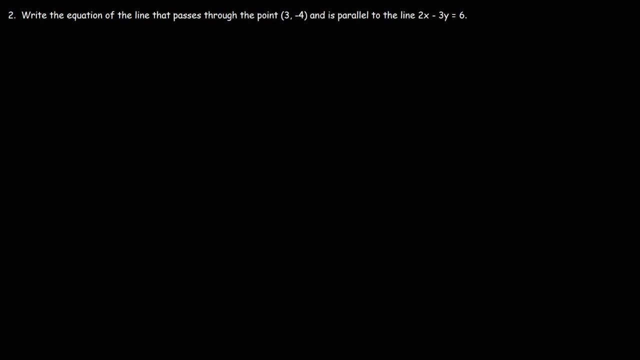 problems. Here's another one. Write the equation of the line that passes through the point 3, comma negative 4 and is parallel to the line: 2x minus 3y equals 6.. So we have the point of interest: 3 negative 4, x1 is 3, y1 is negative 4, and we're going to use the same formula, the point slope. 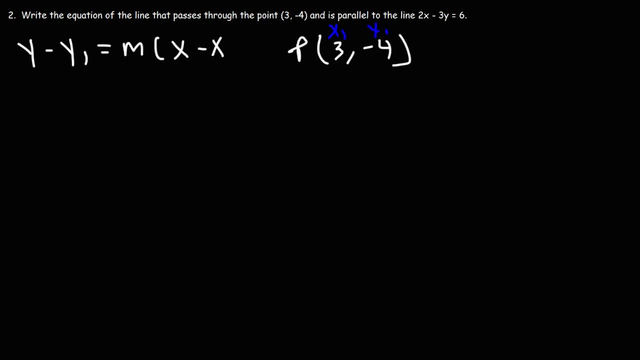 formula to write the equation of the line. So we know x1 and y1.. We need to find m. Now we know that the lines are parallel, so the slopes of the two lines will be exactly the same. The question is: what is the slope of that line? 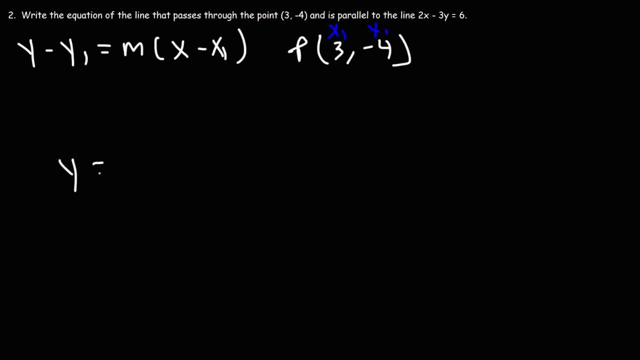 Because it's not in slope-intercept form, It's not in y equals mx plus b form, but rather it is in standard form, that is, ax plus by equals c form. What we need to do if we want to calculate the slope, we need to change this equation from standard form to slope-intercept form. 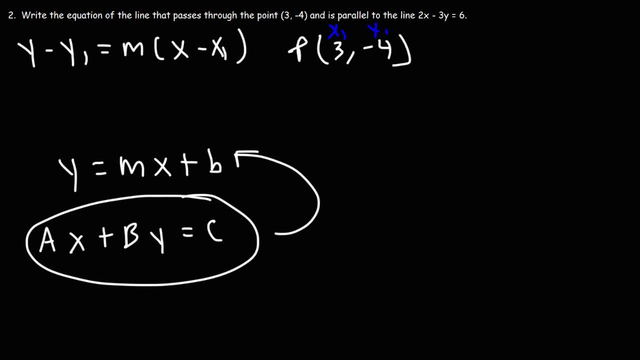 And the way we could do that is by solving for the y variable. If we can get the y variable by itself, we can get the y variable by itself, and we can get the y variable by itself. It's going to be in slope-intercept form, So let's go ahead and do that. 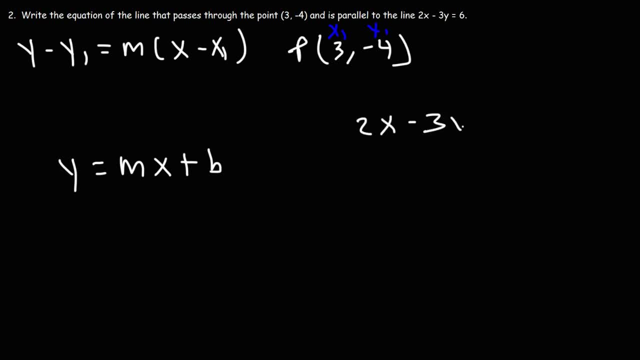 So let's rewrite the equation first: 2x minus 3y is equal to 6.. Now the first thing we're going to do is take the 2x and move it to the other side. It's positive on the left side, but it's going to be negative on the right side. 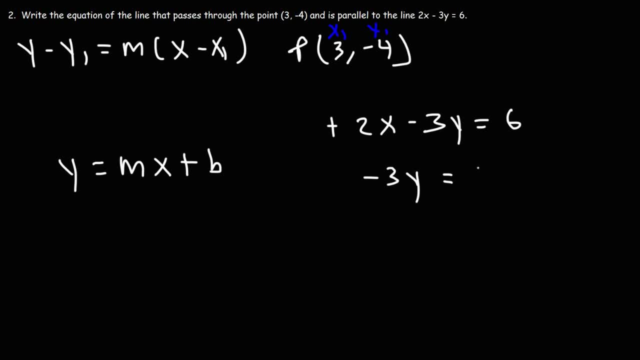 It changes sign when you move from one side to the other. So we have negative. 3y is equal to negative, 2x plus 6.. Next, to get y by itself, divide every term by negative 3. So these two negative signs will cancel and we're going to have: y is equal to positive. 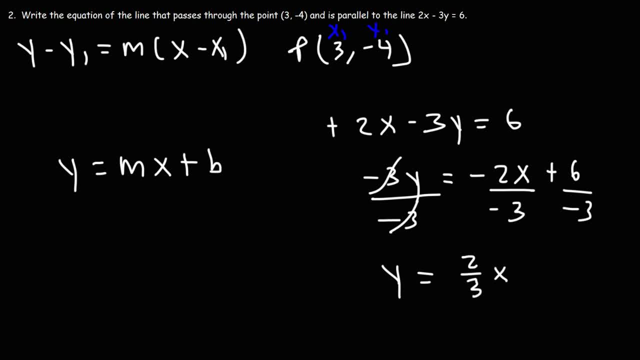 2 over 3x, and then 6 divided by negative 3, that's going to be negative 2.. So now we have the equation in slope-intercept form. We can see that the y-intercept is negative 2, but the slope is the number in front of x. 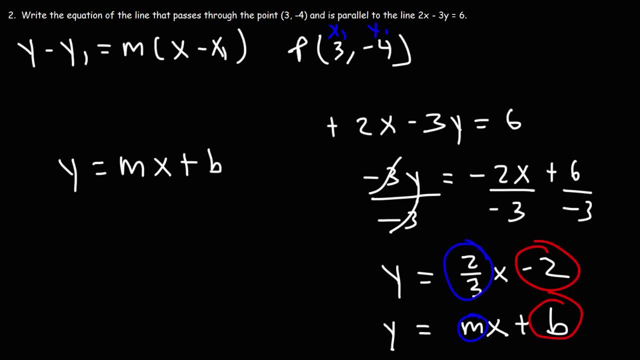 that's 2 over 3.. And that is what we're looking for. So the slope of the line is going to be 2 over 3.. Now we have everything that we need to plug in to that formula, So let's go ahead and do that. Let's replace y1 with negative 4.. 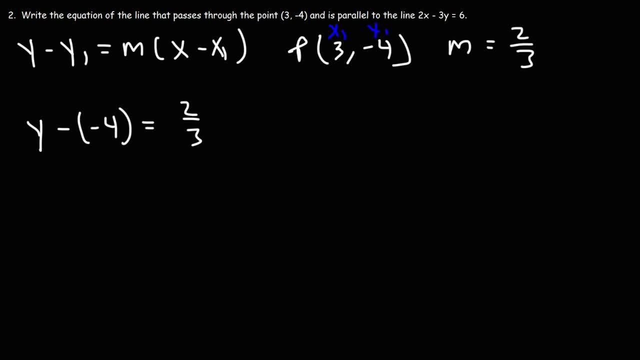 Let's replace m with 2 over 3, and x1 with 3.. So the first thing we can do is change the two negative signs into a positive sign. A negative times a negative is equal to a positive. Now let's distribute the fraction So we have 2 over 3 times x, and then 2 over 3 times negative 3.. 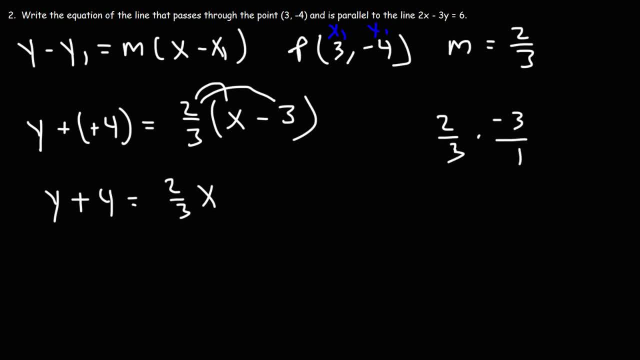 If we multiply these two things, the 3 times negative 3 is equal to negative 3. So we have 2 over 3 times x and then 2 over 3 times negative 3. The 3's will cancel and we're going to get negative 2.. 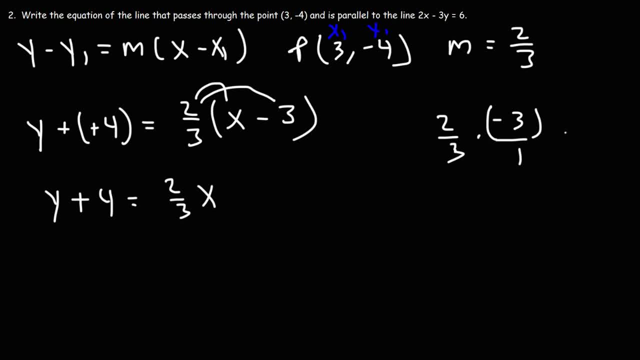 Or you can see it this way: 2 times negative 3 is negative 6, and 3 times 1 is 3. Negative 6 divided by 3 is negative 2. Side the case, the 3's cancel and you get the 2 with the negative sign in front of it. 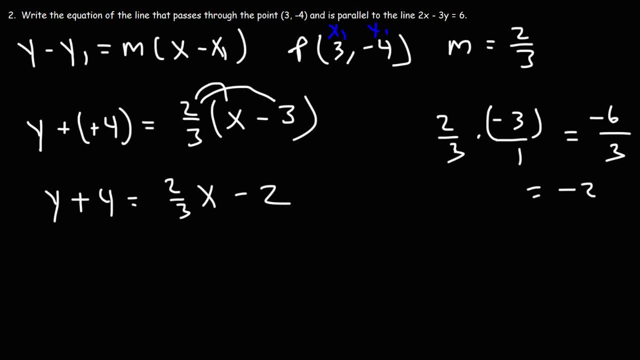 So this is what we now have. Our next step is to subtract both sides by 4. And so we get our answer. in slope-intercept form, y is equal to 2 over 3x minus 6.. So because the lines are parallel, the slopes are the same. 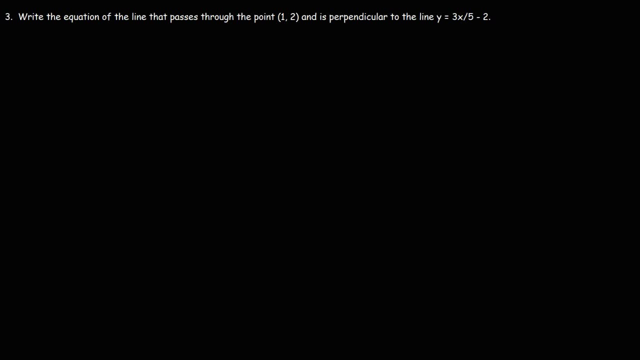 Now let's move on to our last question. Write the equation of the line that passes through the point 1, 2 and is perpendicular to the line that passes through the point 1, 2.. To the line, y equals 3 over 5 times x minus 2.. 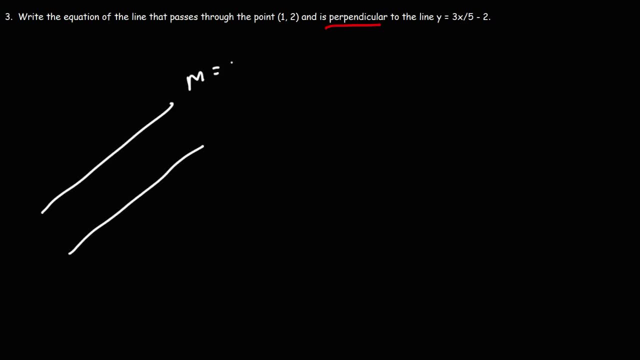 So we know that if two lines are parallel, the slopes are the same. Let's call this line A and line B. So when you see this symbol, it means that the two lines are parallel. Now what about if they're perpendicular? Let's say, this is line A and this is line B. 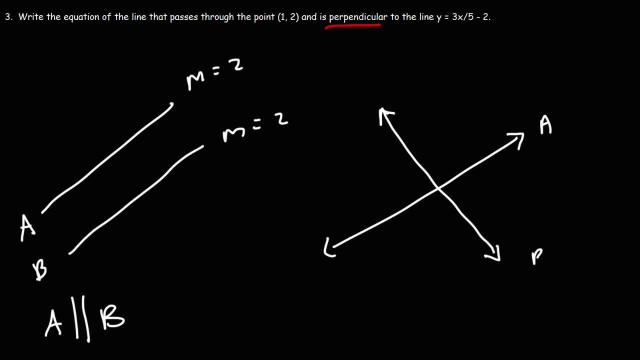 Let's say this is line B. Let's say this is line A. Perpendicular lines, they meet at right angles. There is a 90-degree angle between them And we could represent that using this symbol. So if you were to see this symbol, it tells you that the two lines are perpendicular to each other. 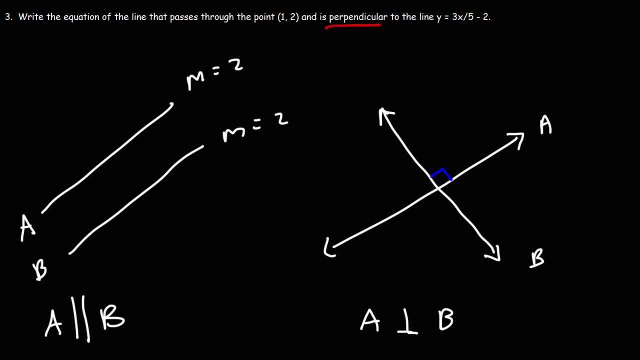 Now the key is to understand how their slopes are related to each other, because the slopes are not the same. Let's say that the slope of line A is 5x4x4.. So the slope of line A is 5x4x4.. 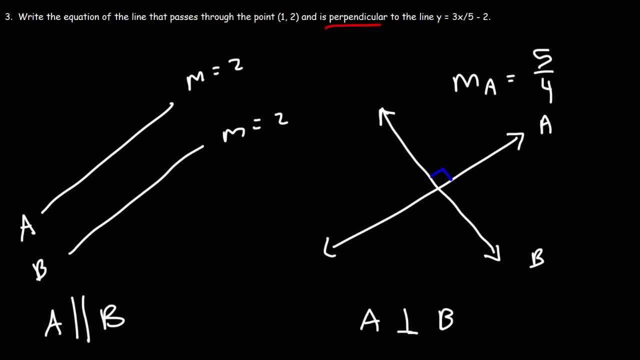 And so the slope of line A is 5x4x4.. 5 over 4.. And let's say it's positive because that line is going up. We can determine the slope of line B If the slope of line A is positive, 5 over 4,. 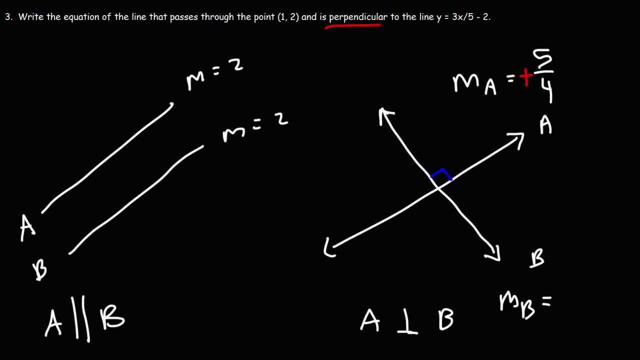 the slope of line B is going to be the negative. reciprocal of that, We're going to change the sign from positive to negative and then we're going to flip the fraction, So instead of it being 5 over 4, it's going to be 4 over 5.. 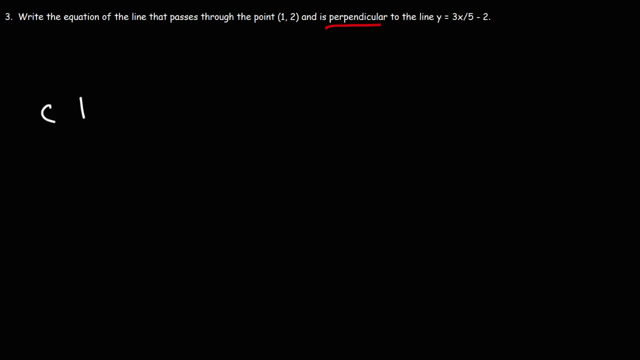 So let's look at another example. Let's say that C line C is perpendicular to line D And the slope of line C- we're going to say it's negative, 7 over 5.. If these two lines are perpendicular, then the slope of line D is going to be positive. 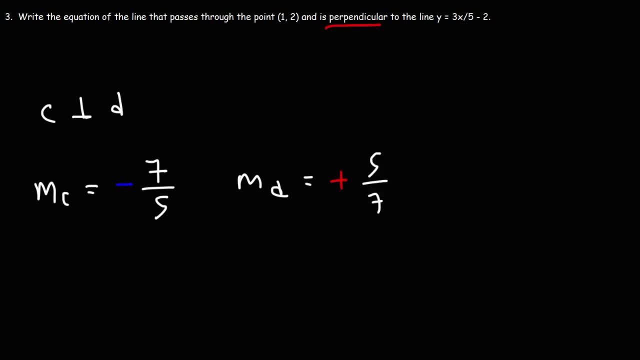 5 over 7.. So you need to find the negative reciprocal of the slope. So you change the sign and flip the fraction. Now let's focus on this problem. So we want to write the equation of the line that's parallel to this one, So the slope, 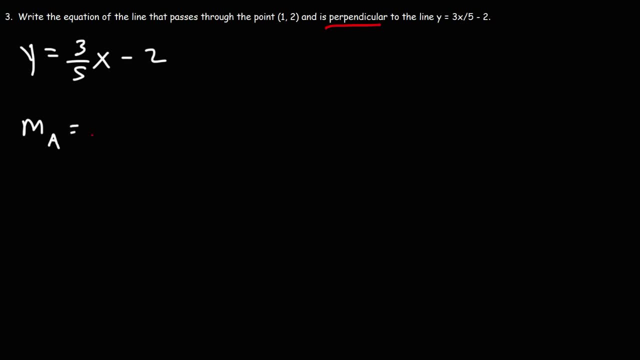 of this line- let's call it line A- is positive: 3 over 5.. The slope of the line that we're trying to find- let's call it line B- that's going to be negative, and then we need to flip the fraction 5 over 3.. So this is: 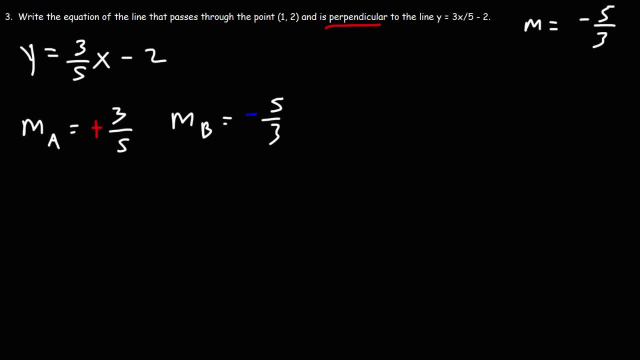 the slope that we're going to use in the formula. So let's write our point-slope formula: y minus y1 is equal to m times x minus x1.. And we want the equation that passes through the point 1 comma 2.. 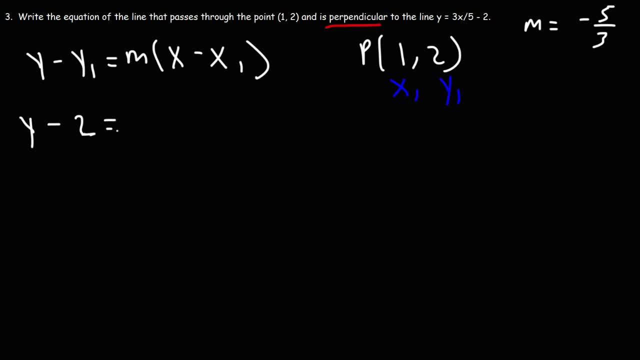 So y1 is 2, m is negative 5 over 3, and x is 1.. So let's distribute the fraction. So this is going to be negative 5 over 3 times x, and then negative 5 over 3 times negative 1, that's positive 5 over 3.. 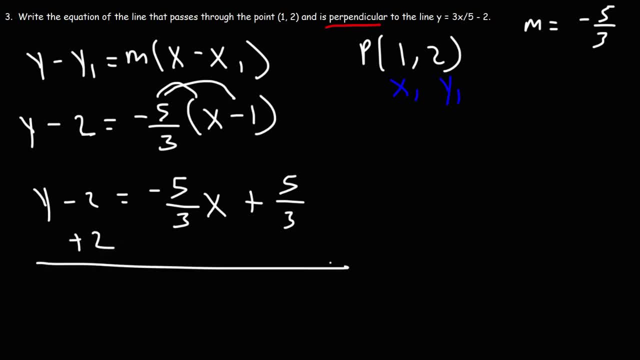 Now let's add 2 to both sides. So right now we're going to have: y is equal to negative 5 over 3x plus 5 over 3 plus 2.. Now 2, I'm going to change that into a fraction. 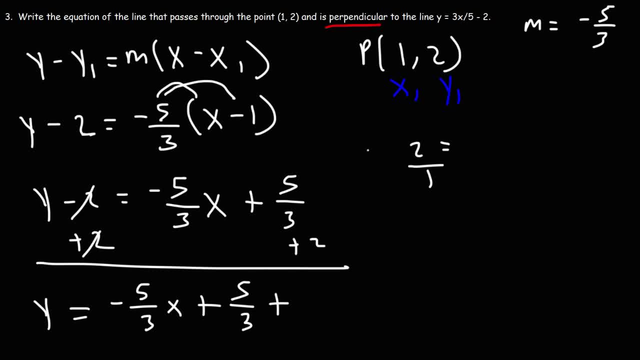 2 is the same as 2 over 1.. And if we multiply the top and the bottom by 3 over 3, we get 6 over 3.. So 2 is the same as 6 over 3.. 6 divided by 3 is 2.. So I'm going to replace the 2 with 6 over 3.. 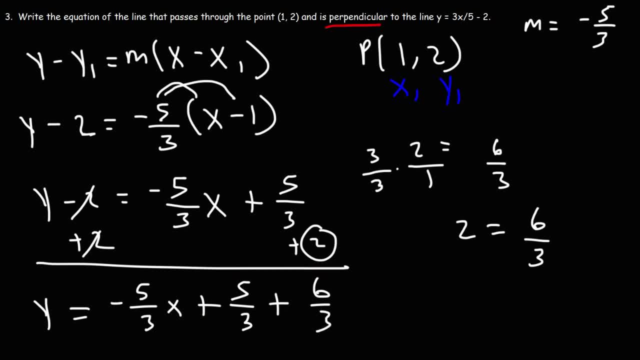 Because now I can add the two fractions, since they have the same denominator. So 5 plus 6 is going to be 11.. So this is the equation of the line that passes through the point 1, 2, but it's perpendicular. 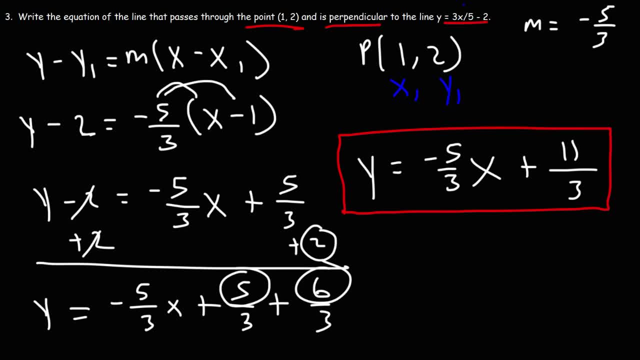 to this line. As you can see, here the slope is positive 3 over 5.. Here it's the negative reciprocal of 5. It's negative 5 over 3.. And we can also check our work by plugging in the point 1, 2.. 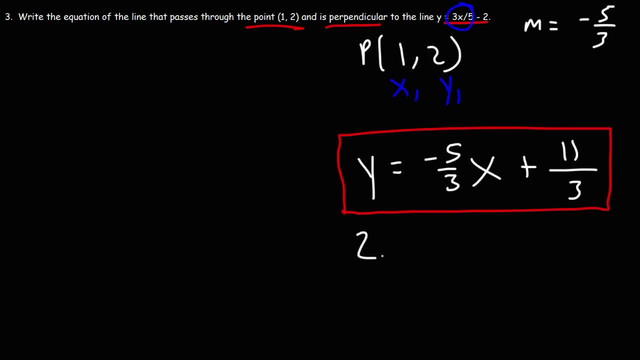 So if we replace y with 2, and if we replace x with 1,, if both sides of the equation are equal to each other, then we know that we have the right answer. So negative 5 over 3 times 1 is just negative 5 over 3..